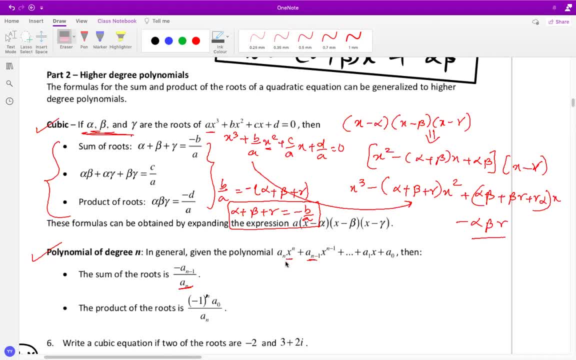 it's a degree five polynomial. so here, if you have like, let's say, degree five, this will be degree four is nothing but the coefficient of degree four. so minus b over a. so this is how you do the sum of the roots for all. so some of the root is now going to change. it is irrespective of any degree. 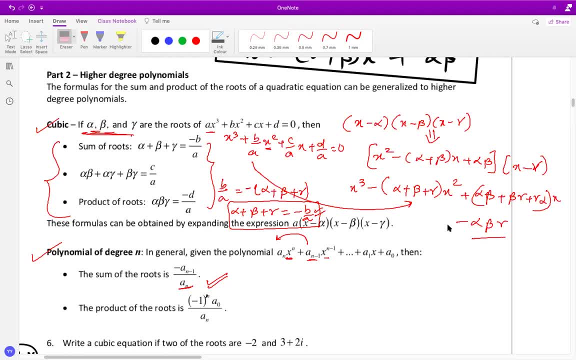 polynomial, it's minus b over a, always. Now, second part is: if you look at the coefficient of x here, so that is c over a and that is equals to this. so alpha, beta plus beta, gamma plus gamma, alpha equals to c over a. and the last part is this: which is d over a, which is: 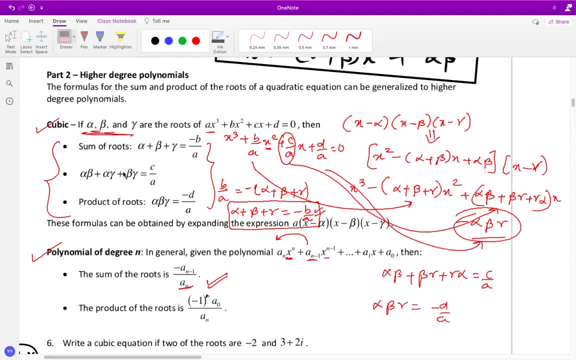 alpha beta gamma is minus d over a. so that's what we wanted to prove and you've got to remember this as well. now, just coming back to the higher order polynomial, in case, if it is degree n polynomial, what we do is here: the sum of the root is minus b over a, but product of the root is alpha beta. 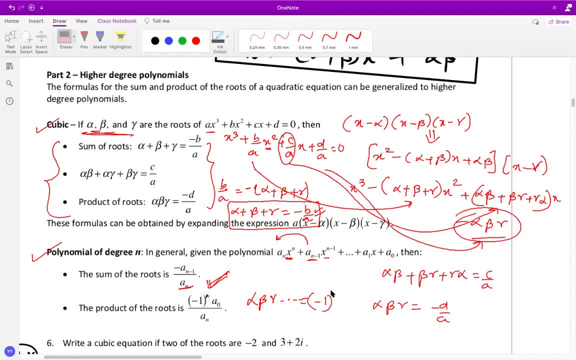 gamma and so on, is nothing but minus one to the power n. a naught over a- and that's a naught- is the constant term, or a, and that's the high leading coefficient. so it's like, for example, if it is cubic, this is going to be odd, so that's why you're getting minus here. so minus d over a if it was. 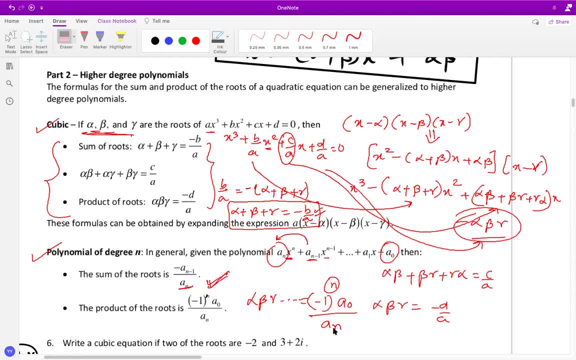 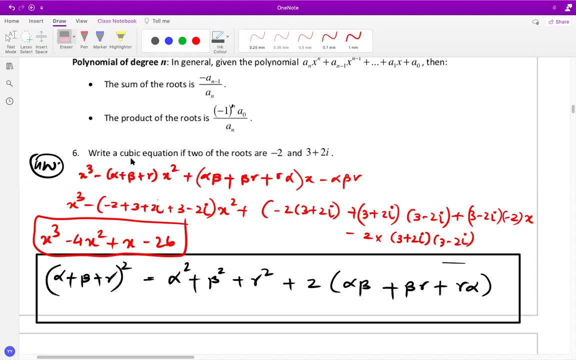 quadratic polynomial it will be. even so in that case will be a naught over a n. so this is just the basic concept and now let's go over some problems. Now the first example is: let's say, if you want to form a cubic equation whose roots are negative two and one of the other root is the, 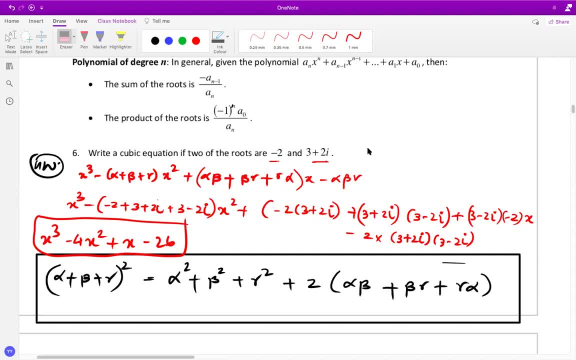 complex root, so three plus two i. and by the principle of the roots concept, if you know that the other root will be conjugate of this, which is the root of the complex root, so three plus two i. and by the principle of the roots concept if you know that the other root will be conjugate of this. 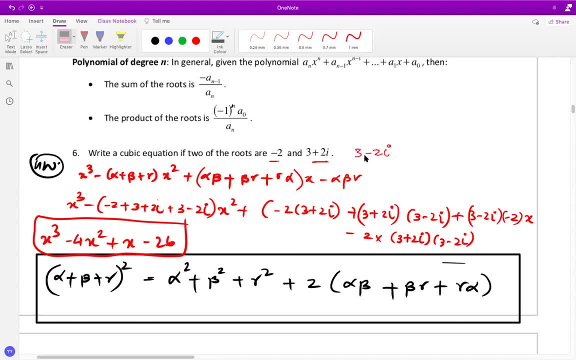 conjugate is nothing but three minus two i. you get the conjugate by just making the sign of imaginary part opposite to what it is, so that there are three roots. these are the three roots, and now, when you want to get a cubic equation, you can just simply use this formula: 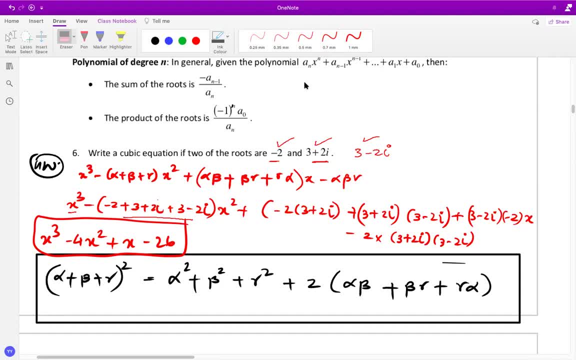 x cube minus sum of the roots. like here, what i'm doing is i'm just doing the sum of the roots times. so this is the sum of the roots part which is here. this is the sum of the roots. so first root is this, second root is this and third, so add them up, that's the coefficient of x squared. 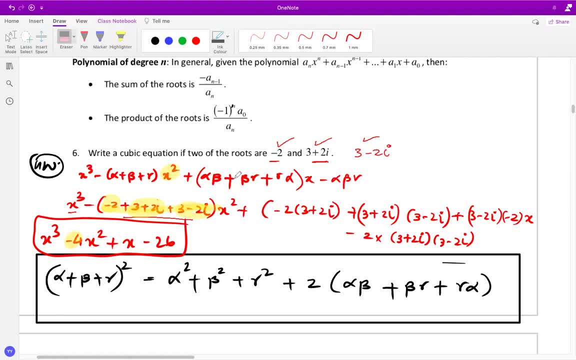 so that is that simplifies to negative four, then product of the root, two taken at a time, so alpha, beta, so this times this, then this times this, and then this times this, and sum of that that becomes a coefficient of x and eventually the last one is the product of the root, which is negative alpha. 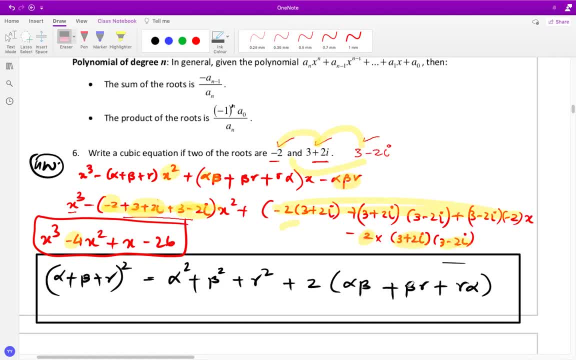 beta, gamma. so negative alpha, beta and gamma. and if you simplify all these expressions you get a get a quad cubic equation like this, which is x cube minus 4x squared plus x minus 26. so this is this simplification. i can just show it to you quickly here. so let's say i have got negative two. 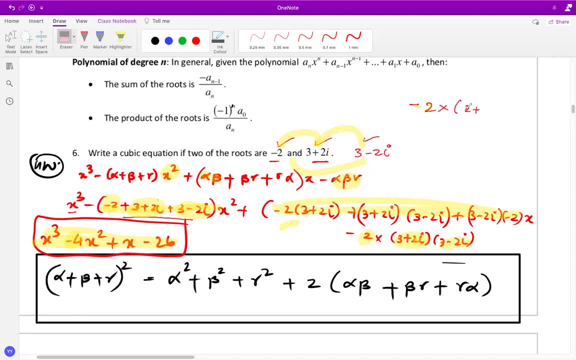 um, let's say negative two times three plus two i times three minus two i, so it'll be negative two times nine um minus two i squared, so that'll be negative two times nine plus four. so nine plus four is thirteen. thirteen times there is negative 26.. so that's how you're getting the value of the. 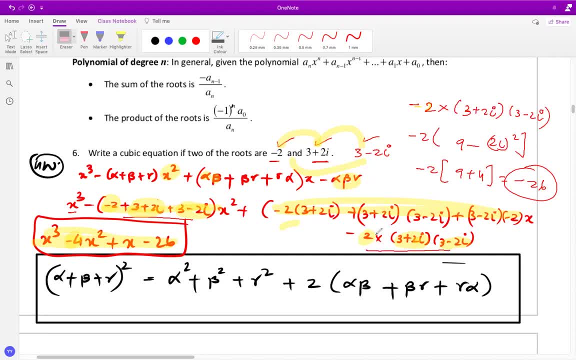 cons the product as negative 26.. so negative 26. and because this value is negative 26, so negative times negative x will become positive 26.. so that's how you do the like. you form the equation when you have been given the roots. so when you simplify these parts, let's say this part is going to be negative 26, so obviously, 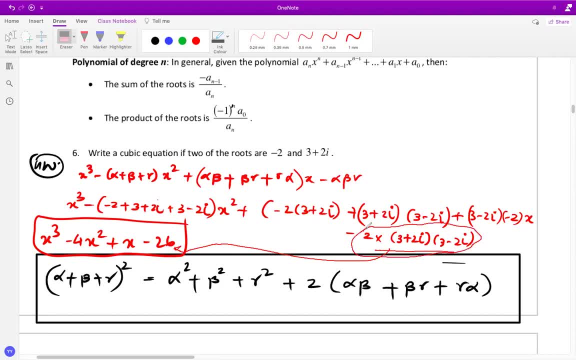 this entire thing that you get here is two times. this thing is positive, 26 times negative. so that's how you get negative 26.. and these terms, when you simplify that, is going to come to positive 1x, and this one, if you simplify this, negative 4. and so this is how you get the. they get the cubic equation. 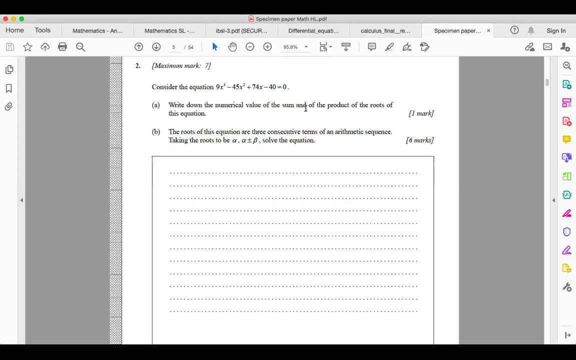 so now here the question is: write down the numerical value, the sum and the product of the roots of this given equation now, since it's a cubic equation that we can see here. so the sum of the roots that we get is alpha plus beta plus, let's say, gamma is. 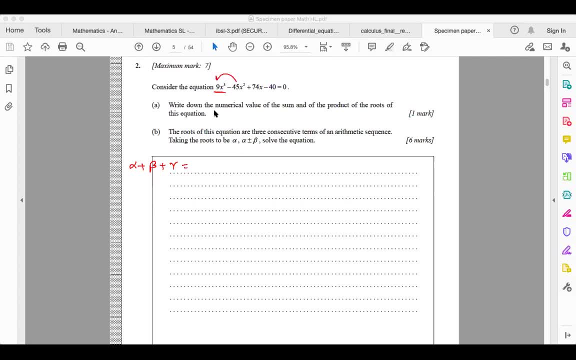 um here of minus b over a, so that's going to be negative, of b, which is minus 45 over a, which is 9. so that's sum of the root is 5.. product of the root is alpha beta. gamma is minus c over a, so minus. 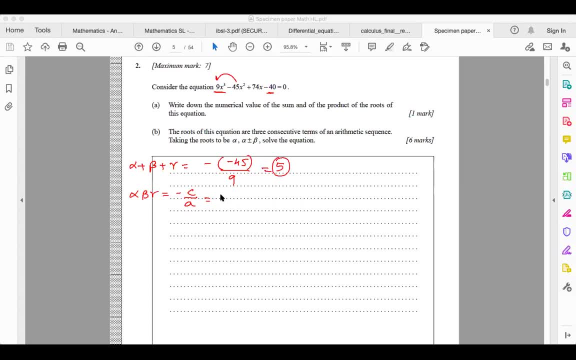 c over a, so that's here. c is negative 40, so it'll be negative of negative 40 over 9. so it's the product of the roots: 40 over 9.. now what they're asking is for the b part, the roots of the equation. 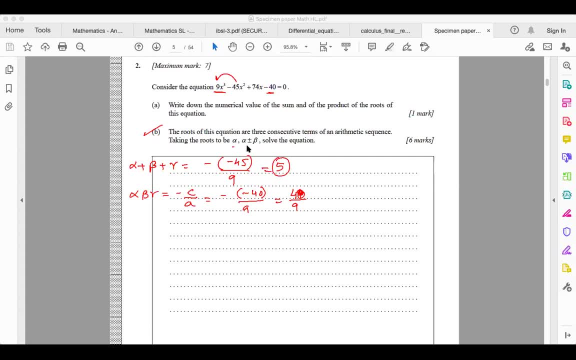 are the three consecutive terms, and and take these roots of alpha, alpha plus beta, alpha minus beta, um the roots of this equation, so you have to find out the value of alpha and beta basically here. so this is um. what we do is that, if you, if you simply look at now, if i take one of the root of alpha plus, 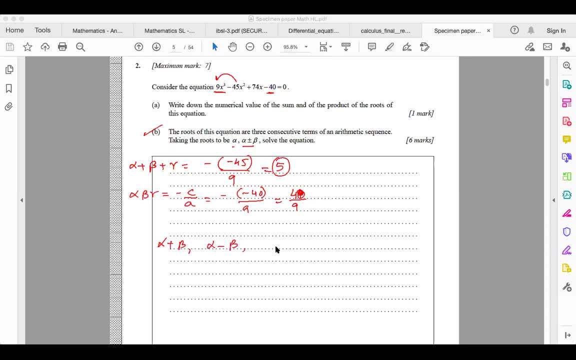 beta, other is alpha minus beta and third one is actually alpha plus beta. we take like this: uh, either alpha minus beta at a, then you take alpha and alpha plus beta. so this is like proper order of the roots and this sum is actually equals to five. so we get some. this sum equals. 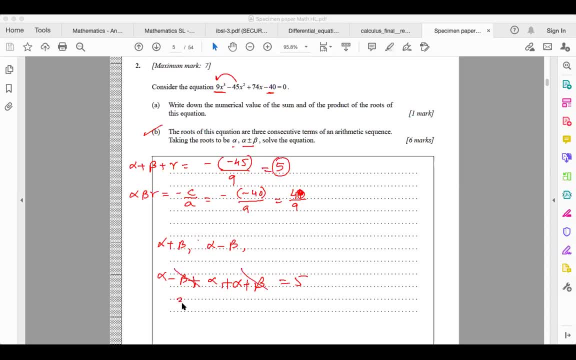 to five. so this you can see that minus beta get cancelled and you get three. alpha is five, so alpha is pi over three. once you get this, uh, second part is the product of the root, so we can use this product of the roots. so now five over three, plus beta times uh, alpha times uh, so alpha. 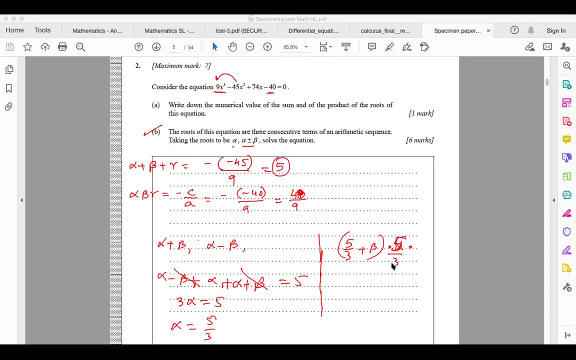 we, we already got which is five over three. so five over three here as well, times uh, five over three minus beta. let's say this equals to forty over nine. so this three and three get cancelled here. so you get five, uh and eight. so you get five over three plus beta. five over three minus. 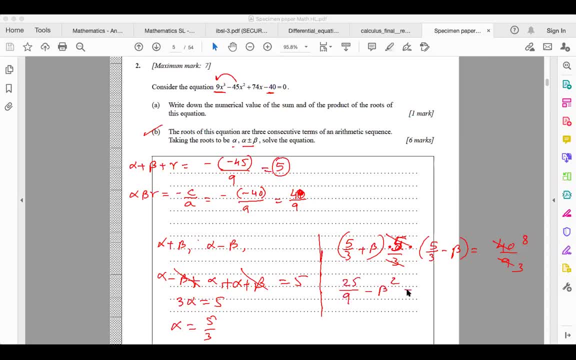 theta, which becomes 25 over nine minus beta square, is eight over three. so after this you solve for beta value. so beta squared is going to be 25 over 9 minus 8 over 3, which is nothing but 25 minus 25. if you multiply this by three and this by three, you get one over, uh, nine as beta squared, so that